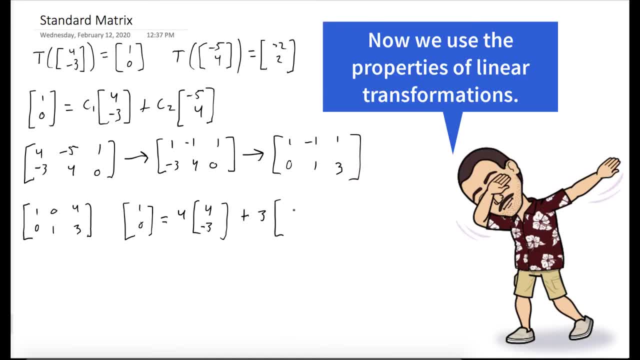 4 times 4, negative 3 plus 3 times minus 5, 4.. So our transformation maps 1, 0. the same way, it maps 4 times 4, negative 3 plus 3 times minus 5, 4.. 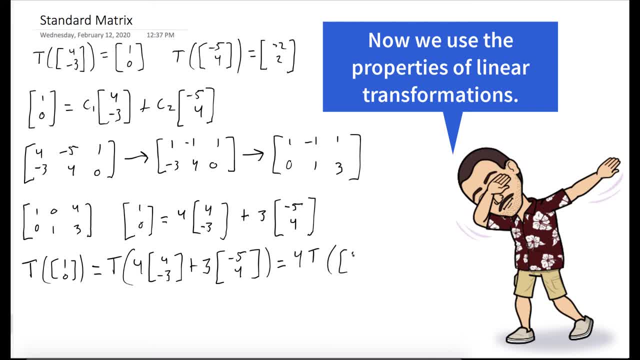 Well, T is a linear transformation, So we could pull out the scalars and break apart the sum And we see that T of 1, 0 is 4 times 1, 0, plus 3 times negative, 2, 2, which is negative. 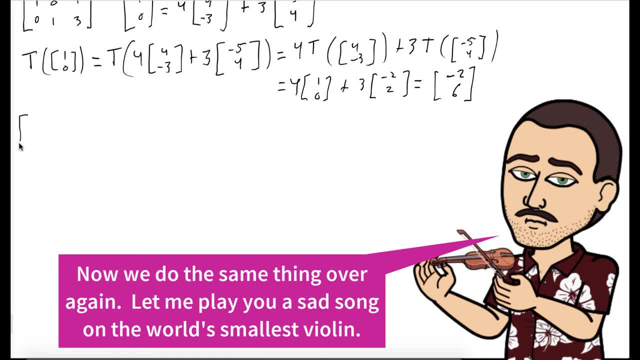 2, 6.. And what we'll do now is do the same thing with the next elementary column, vector 0, 0, 1.. We want to express 0, 1 as a linear combination of 4, negative 3, and minus 5, 4.. 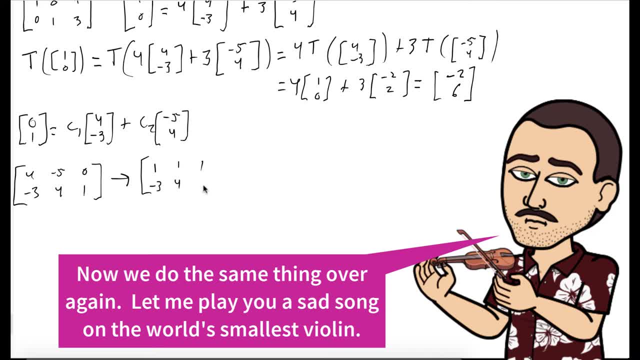 So again, we set up an augmented matrix and row reduce until we can't row reduce anymore. A lot of the steps will be similar as the row reduction from before. And we see we can express the vector 0, 1.. And we see we can express the vector 0, 1 as 5 times 4, negative, 3 plus 4 times minus. 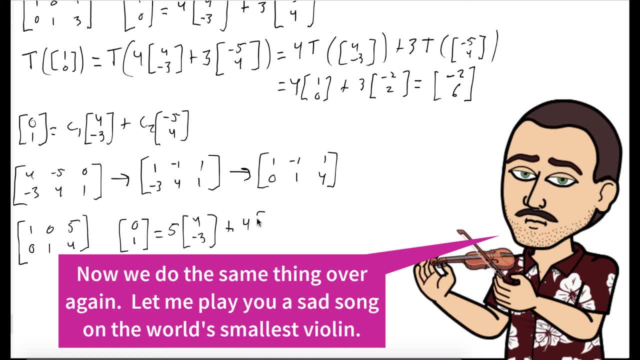 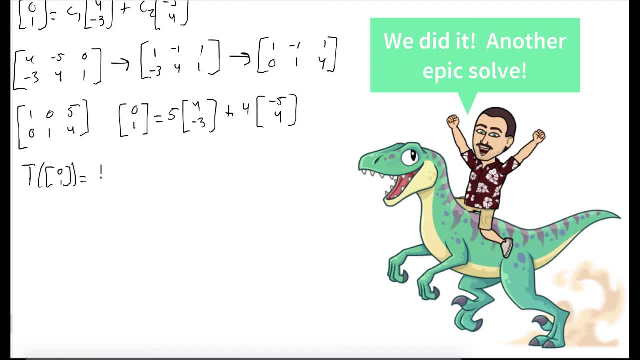 5, 4.. So, as with before, we evaluate the transformation to both sides of this equation. And again, T is still a linear function. So we can break apart this summation and pull out the scalars And we can move on to the next step. 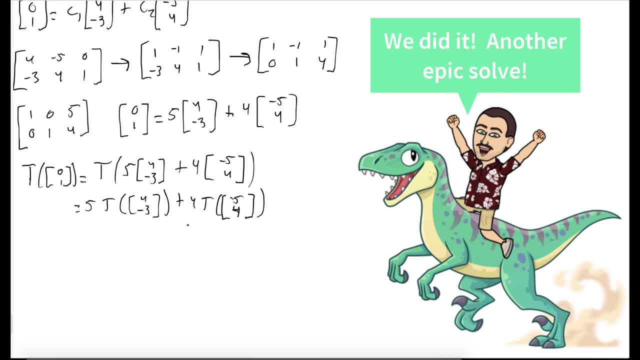 And so we get 5 times 1, 0, plus 4 times minus 2, 2,, which is negative 3, 8.. And so we can conclude that A is negative 2, 6,, negative 3, 8.. Ouch, Don't text and drive Bye-bye.